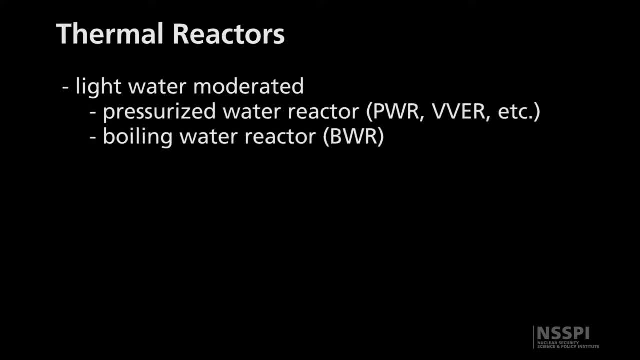 light water moderate reactors. there's principally two types: what's called the pressurized water reactor and the boiling water reactor. The pressurized water reactor, or PWR, is what we principally have here in the United States, though there are also boiling water reactors in the 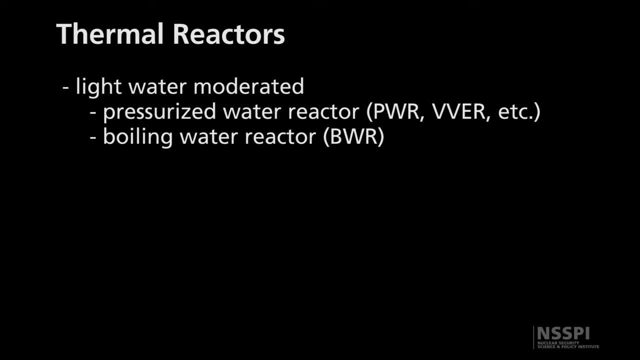 United States as well. The Russians also have a type of pressure water reactor called a VVR, which is generally very similar to the US PWR. There are also heavy water moderated versions of thermal reactors, which use heavy water, which is a type of water that contains deuterium instead of regular. 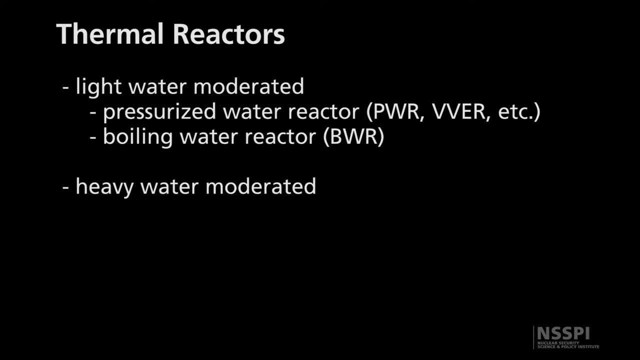 hydrogen And deuterium actually has a mass about twice that of hydrogen. The most common kind of that is a kind of reactor that is called the can-do reactor, which is a type of water that contains deuterium, which is a Canadian-designed reactor that uses a heavy water moderator and a 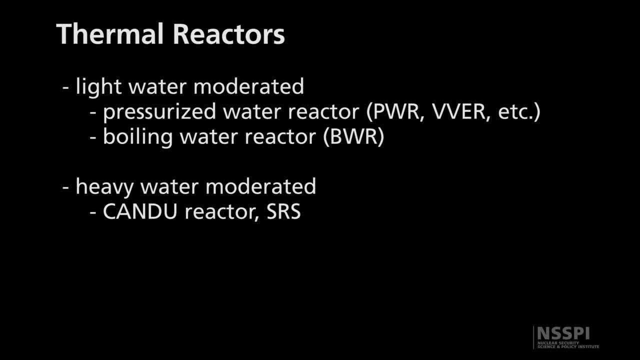 natural uranium fuel. There are also thermal reactors that use graphite as their moderator. In that case they have a solid moderator of graphite and then they either have a gas coolant or a light water coolant to cool the fuel. Of the fast reactor types, there's really only one type, that. 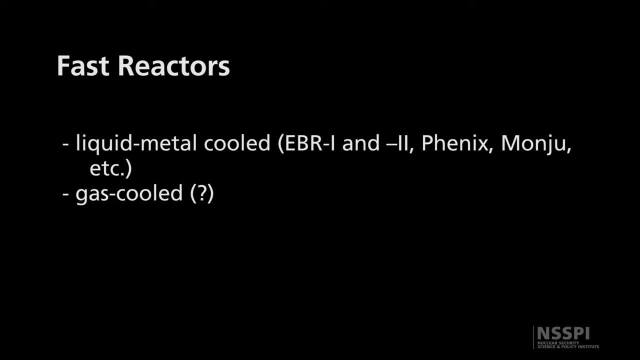 truly exists, which is the liquid metal type reactors. There have been several liquid metal cooled reactors: EBR-1 and EBR-2 were ones in the United States, Phoenix and Phoenix, France, and then Manju in Japan. And of course the Russians also have a set of liquid metal cooled. 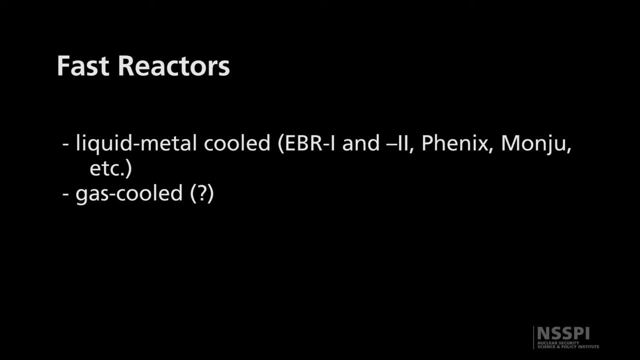 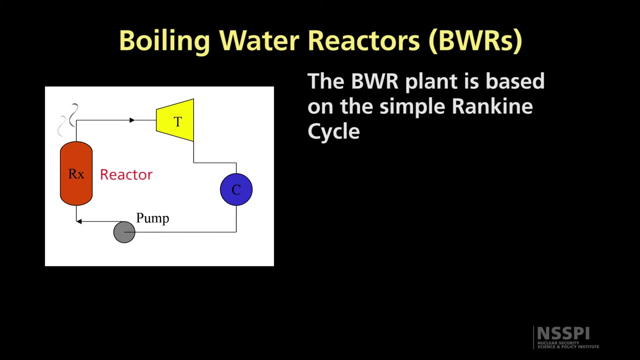 reactors called the BN series reactors. The gas cooled fast reactors is a type that has been designed but really hasn't seen much in the way of production in the world. The BWR reactor, a boiling water reactor, is a very simple reactor type. In this case, the reactor produces steam. 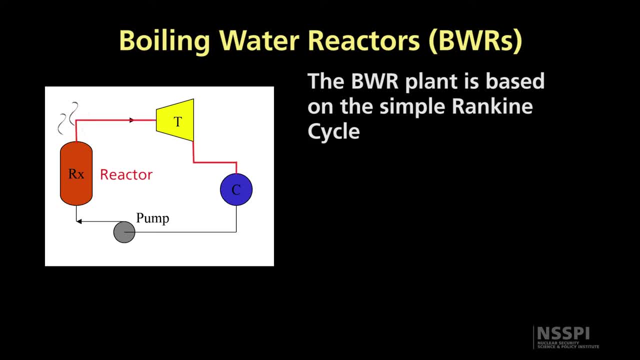 That steam then drives a turbine. The steam then gets condensed in a condenser and pumped back up and throws the reactor. So the cycle for it, the thermodynamic loop for it, is very simple. This reactor operates off of a low pressure light water coolant. It has a low enriched uranium or LEU oxide. 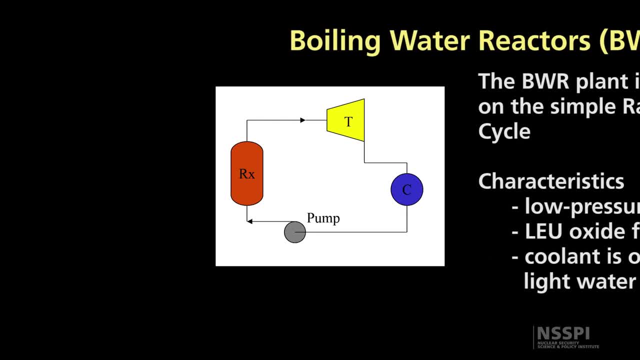 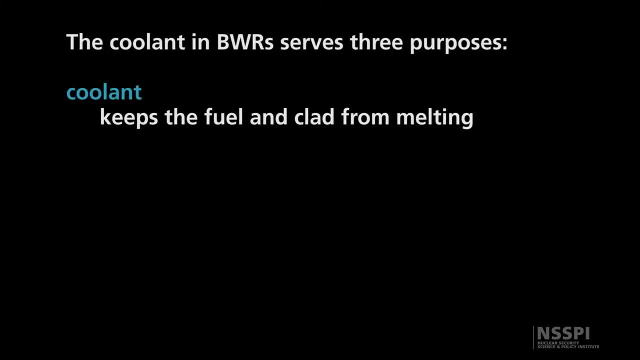 fuel and the coolant is just ordinary light water. The coolant itself serves really three purposes, two of which we've already talked about. It's the coolant to cool the fuel and clad so that keeps the fuel from melting. It's also the moderator that slows the neutrons down. 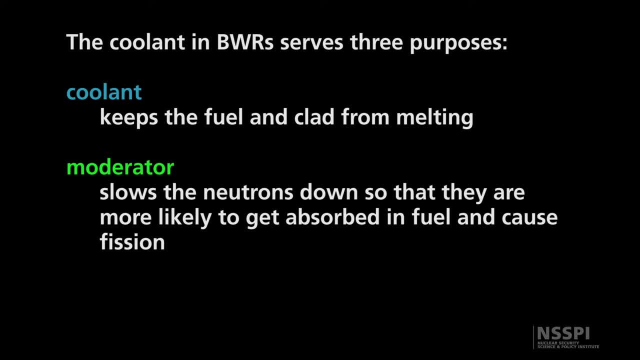 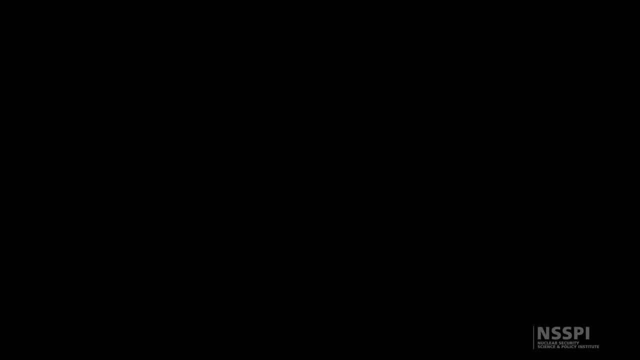 so that they can then get absorbed in the fuel and cause fission. And then it's also the working fluid which then spins the turbine and produces electricity. This type of reactor- BWR reactors- have to use enriched uranium fuel. That's because the coolant 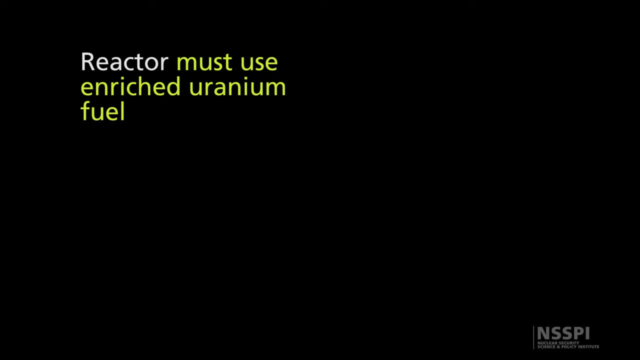 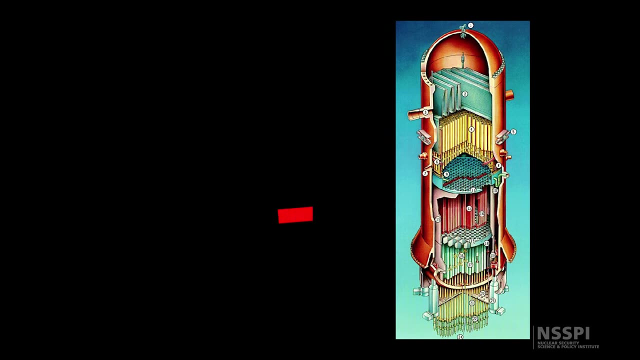 that's used here, which is light water coolant, absorbs a lot of neutrons. It absorbs so many neutrons that you can't use natural uranium. You have to enrich the fuel. This is just internal structures of the reactor itself, where this area here is the actual fuel. The rest of this 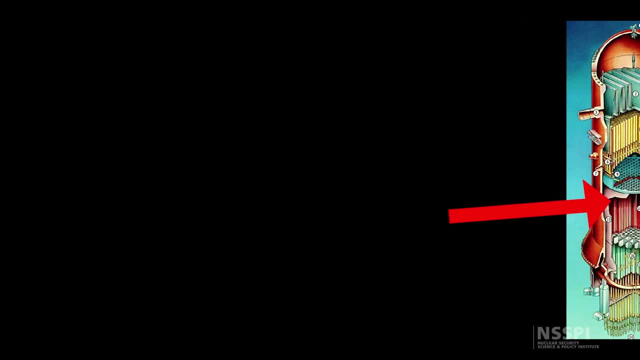 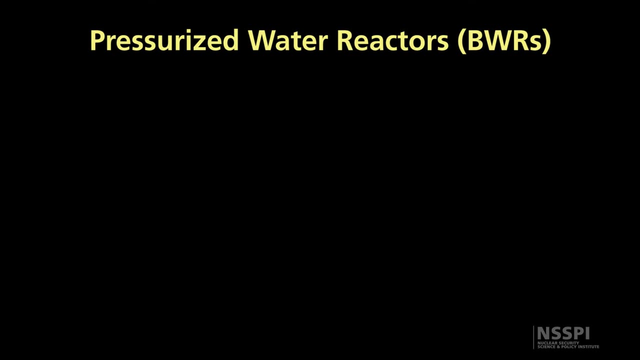 is all control structures and then areas that are used for the coolant system. The pressurized water reactor, or PWR reactor, which is probably the most common reactor system in the world, is slightly more complicated. It actually has a dual loop structure, where it has a primary loop. 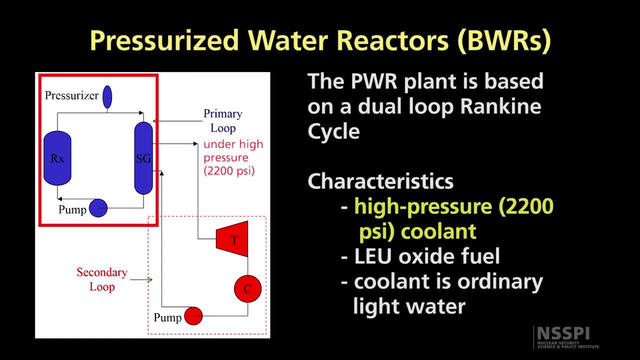 and then a secondary loop. The primary loop is kept at a very high pressure, around 2200 psi. It still uses a light water coolant and it uses a low enriched uranium oxide fuel like the BWR, But this coolant, since it's at a higher pressure, this coolant does not boil, It stays as a liquid. 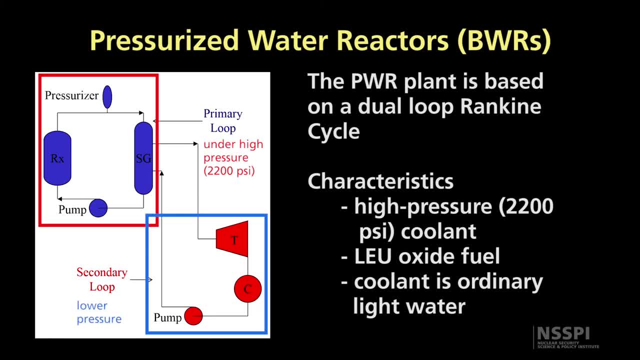 and then the secondary loop is kept at a lower pressure and that coolant then boils in this thing called a steam generator, And then that steam then is used to drive a turbine. The dual loop system allows you to keep any radiation from contaminating the turbine. There's no 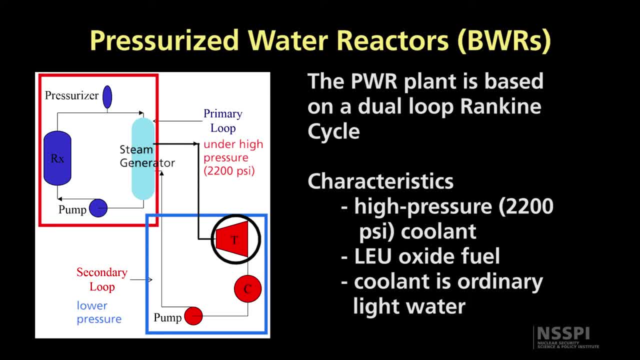 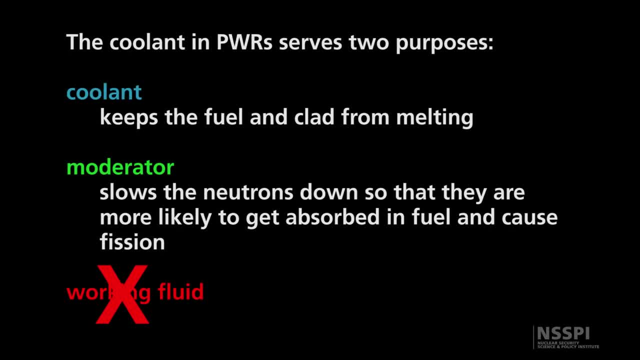 radioactive materials that will go over and contaminate the turbine because it's separated into these two separate loops. The PWR reactor also uses a coolant that serves as the moderator, but that same coolant, that same coolant, is used to keep the coolant from getting contaminated. 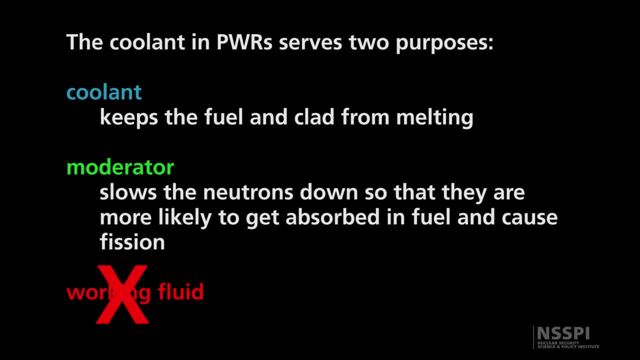 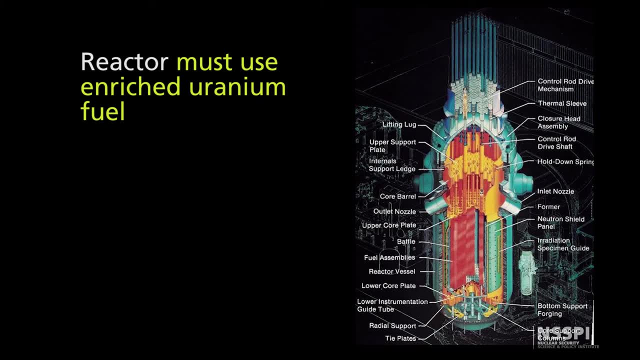 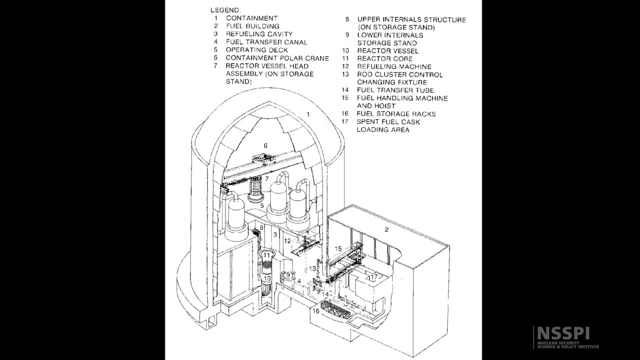 So the coolant for the fuel does not serve as the working fluid. This reactor, since it uses a light water reactor, also has to use an enriched uranium fuel. And again, that's just a picture showing the typical Westinghouse style PWR reactor. This is the structures of the pressurized water. 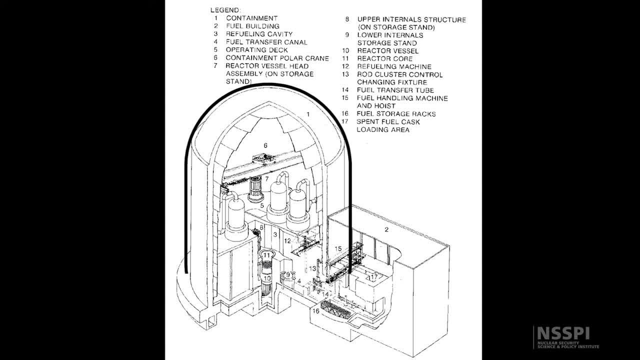 reactor, which is the containment structure that you would expect to see. The reactor is the small little thing right there in the center. The large structures here are actually the steam generators that are being used for the reactor, And then a containment around the outside which is there to 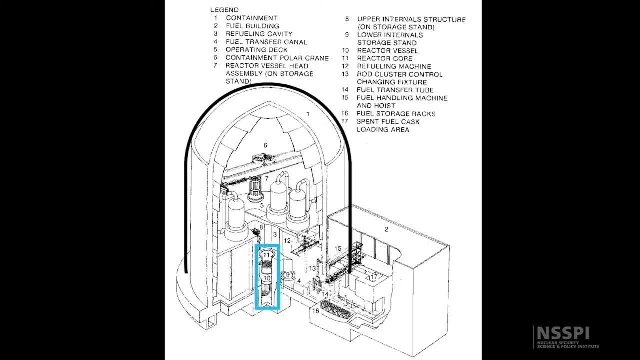 provide safety so that if anything bad happened inside the reactor, that this would all get contained inside of this large concrete and steel structure. Also shown here in this other building is the spent fuel pool, where spent fuel from the reactor is stored in a separate building outside. 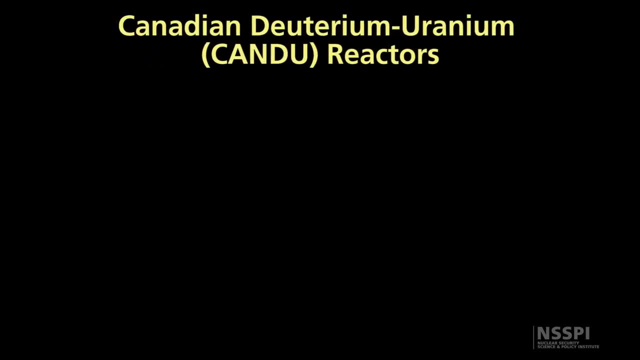 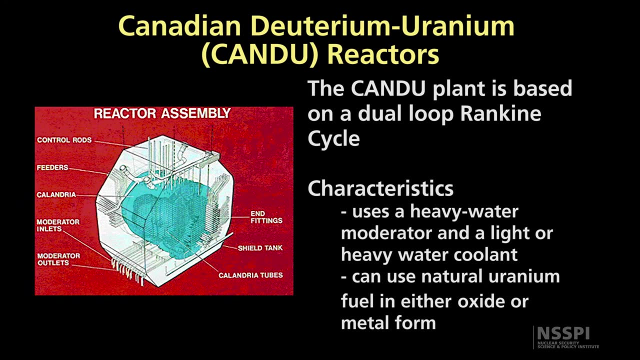 of containment. Another type of reactor that we see in the world is the CANDU reactor. The CANDU reactor was designed by the Canadians. It's based again on a dual loop Rankine cycle, similar in many ways to a PWR. The coolant itself. 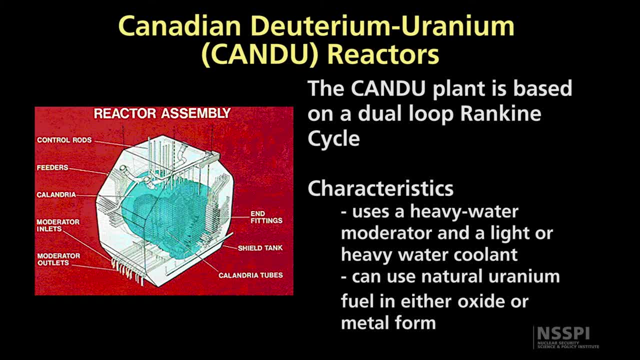 is a either light water or heavy water coolant that flows through a set of pressure tubes in the center of the reactor. So what's shown here is each of these little tubes. here is a pressure tube running through the core, and each tube is an individual tube. Inside of that tube, then, is a 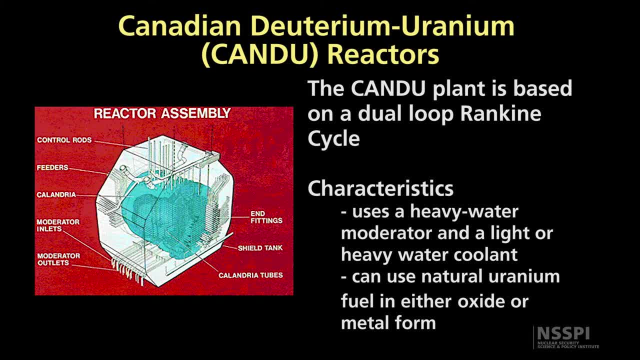 natural uranium fuel, usually in oxide form, but it technically could be metallic form as well. And then in this larger tank around the outside of the reactor there's a pressure tube that's running through the outside. is this heavy water moderator, which is kept at a fairly low pressure? 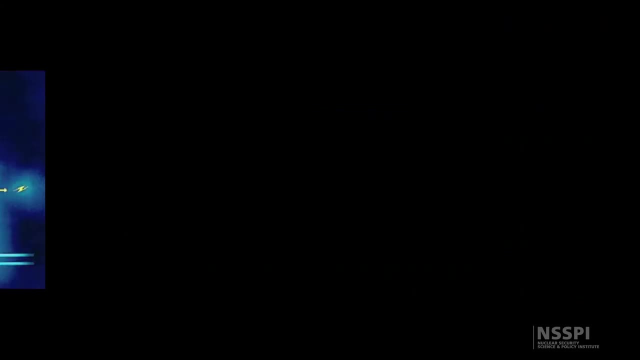 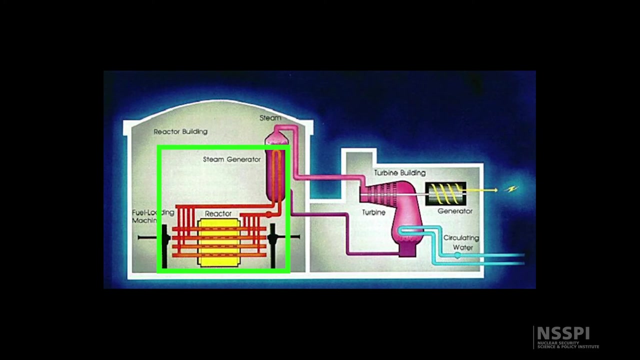 and the heavy water moderator then serves to moderate the neutrons. Like I said, the system is in a dual loop system, so this is your primary loop here, and then that primary loop then produces steam in a steam generator which goes through a secondary loop. 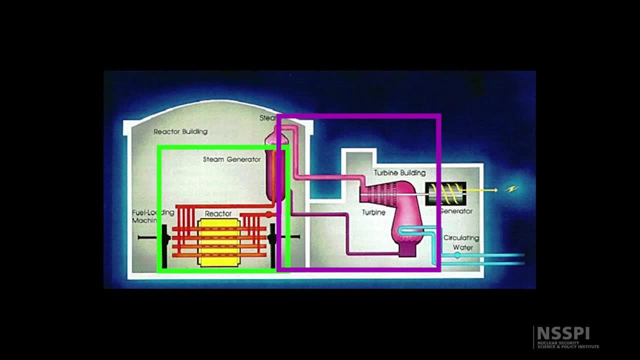 including flow through a turbine to produce electricity. So in that respect, it's fairly similar. One difference, though, you see, is that this reactor is actually on its side- The PWR reactor. the cylinder was up and down. In this case, the cylinder is on its side and the water flows through the reactor sideways. 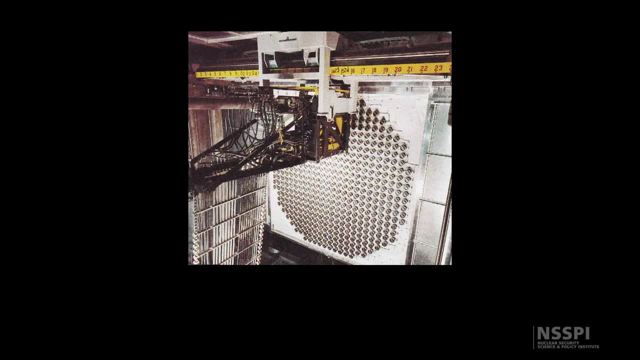 This picture shows the refueling machine of a can-do reactor. One of its more interesting characteristics is the fact that the reactor can be online refueled, So while the reactor is still operating, they can turn off individual pressure tubes and then pull fuel out of those pressure tubes and put new fuel in.